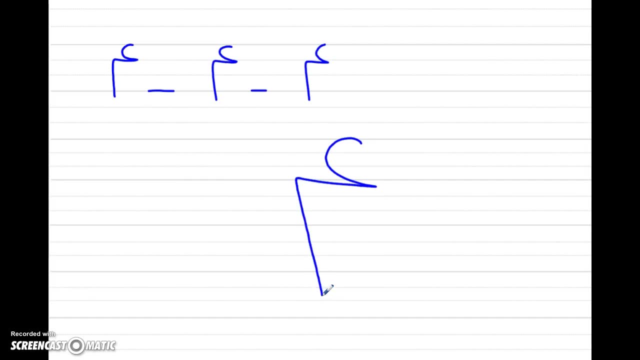 Char, Char, Char. So this is a right angle, But on top of it you have this semi-circle shape. So you make this like a semi-circle, You go and make a right angle, So char, Char, And then this is five, which is like an upside-down heart. 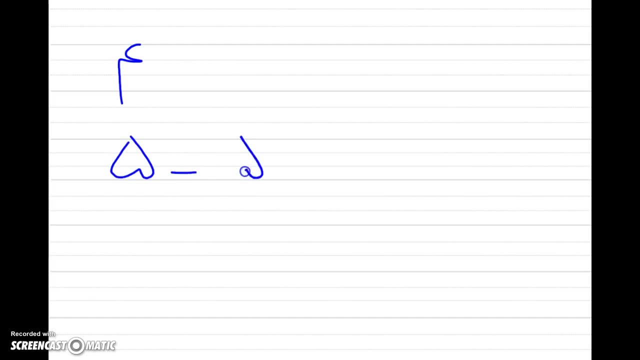 Panj, Panj, Panj, Panj, And then shish, The semi-circle again, but with a slanted line: Shish Shish, Which is six, Shish Shish Halved, Which is seven. 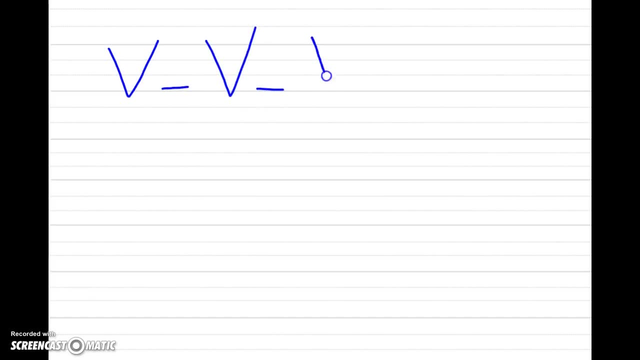 Halved, Just like a V Halved. Now, this part is exactly the V, but it's upside down and it's hashed, which is 8.. Hashed, Hashed, And then 9 looks like English 9, but this is how we write it. 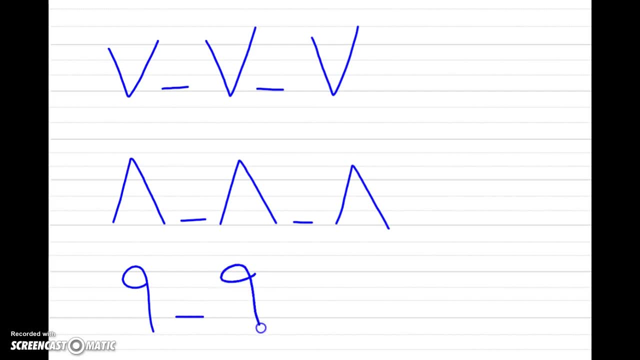 9. No, No, No, No, And then dah a 1, and a 0.. 0 is like just a dot. I made it larger so you can see it, but it's just a dot, like you know, the dots that you have in Farsi. 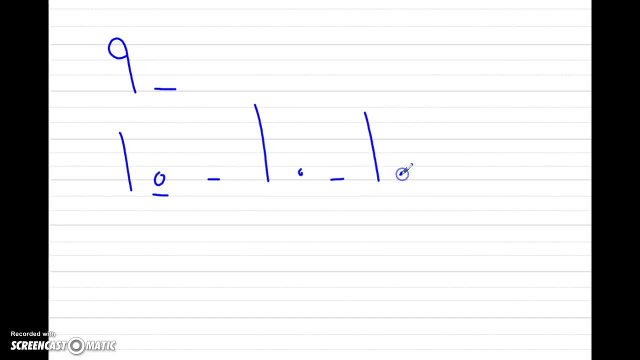 This is dah, Dah, Dah. And then this: This is sifr, Sifr, Sifr. Now we're going to do all of them together: 1., 2., 3., 4., 5., 6.. 7., 8., 9., 10., 11., 11., 12., 13., 14., 15., 16., 17., 18., 19., 20., 21. 22.. 22., 23., 24., 25., 26., 26., 27., 28., 29., 30., 31., 32., 33., 33., 34., 35., 36..